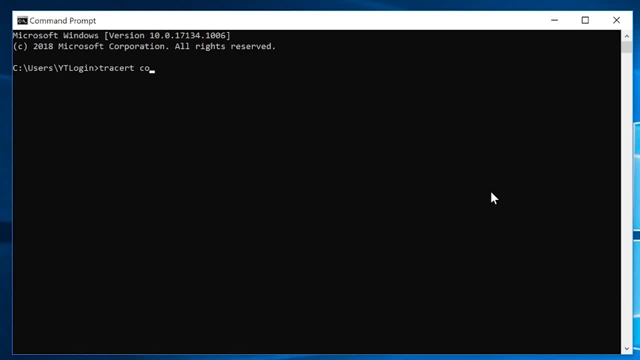 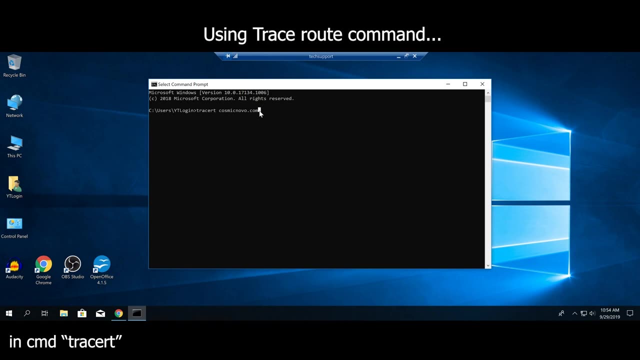 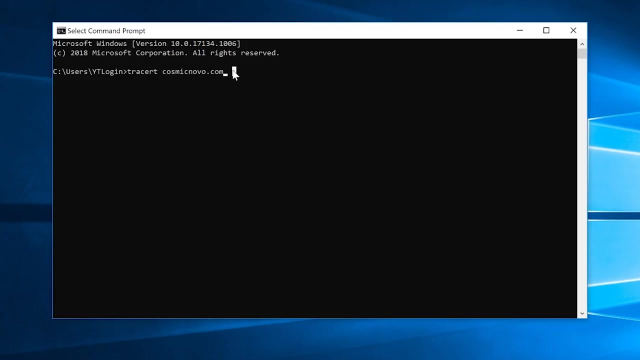 TraceRT, followed by the name of the website you're trying to reach. This doesn't have to be a website. It could be a server of some sort, or a switch, or I should say just an IP address of a network component or a location. So- and that gets me into why would you want to use TraceRT before? 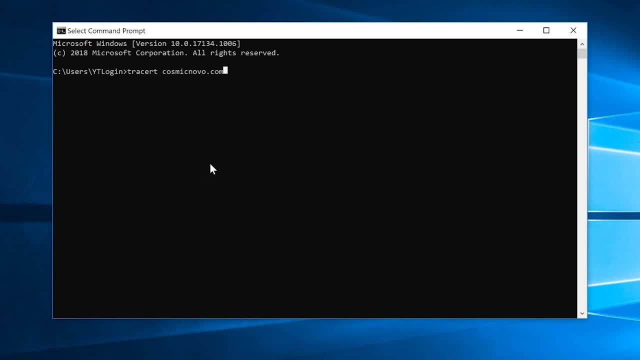 I even hit enter here, and then a bunch of stuff comes up. I want you to understand why you would want to use it. So let's say, at your work, at your office, for some reason, you cannot reach CosmicNovocom, However, from your phone, which is, by the way, on a. 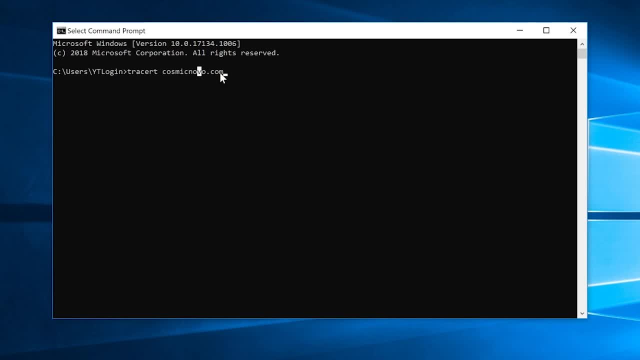 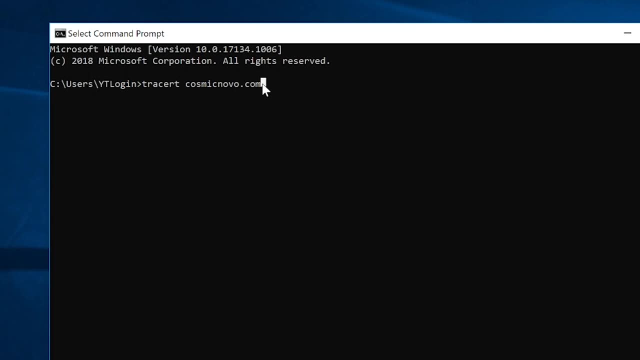 network. on a different network entirely, you can reach CosmicNovo just fine. Also, another example is an application that uses network connection to work, For example, an application that has to reach to a network connection to work. So, for example, an application that has to reach to a network. 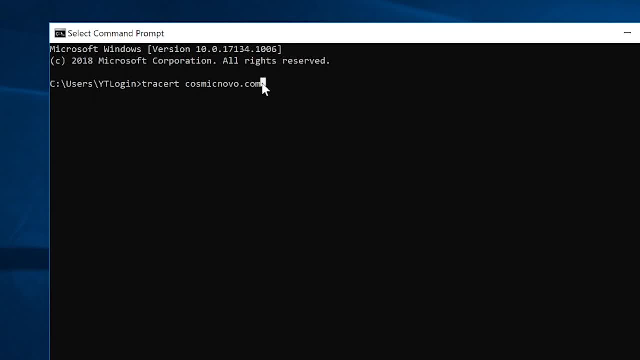 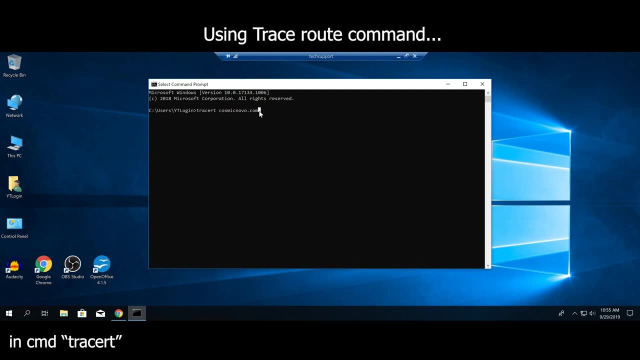 a database that could be located in a totally different state, country this- and that It could be at the end of the world. It could be that it's not working. That's another reason you would want to use TraceRT. Or simply there is a server somewhere we can't reach whether it's used for. 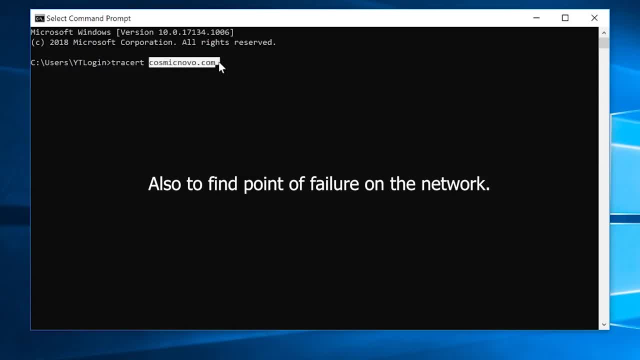 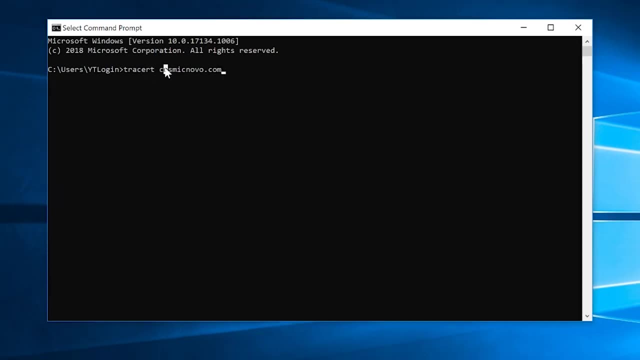 storage or this, and that We would want to use TraceRT to figure out why you can't reach it from your office network, but you can reach it from any other network. So what it does in the nutshell, TraceRT? it traces all the routes taken on the network to reach. 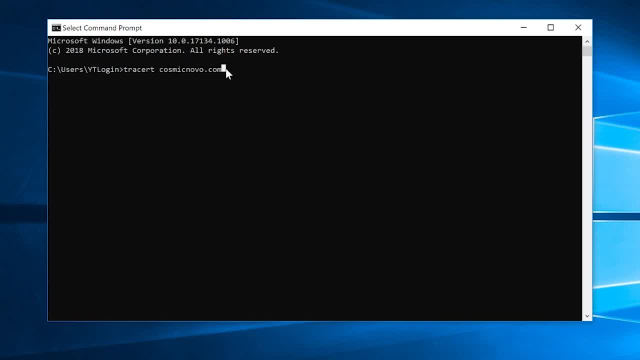 CosmicNovocom in this example, So it's going to map it out for me. So think about it this way. Let's say you have a date or you are going somewhere that you've never been before. You open up your phone, You go to Google or Apple or whatever that you're using. You type in your 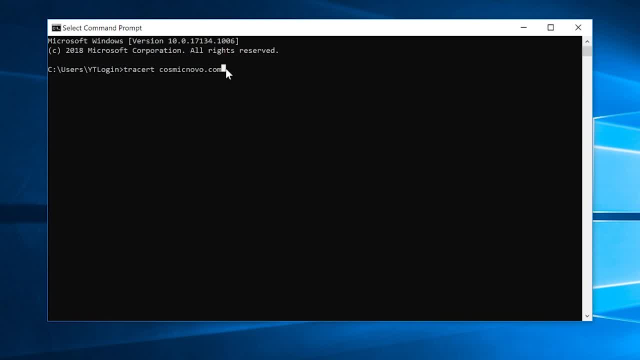 navigation, the address that you want to visit, And it gives you all these routes that it takes. You know, it says go straight, go left, go right, this, and that The TraceRT kind of does the same thing. in a sense, However, TraceRT, it will tell you whether there are certain roads or routes that 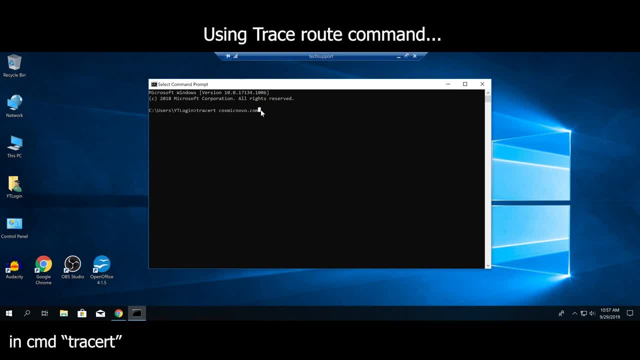 you cannot take, or that they're broken or non-existent. So that's a very simple explanation of what TraceRT does. It tells you whether a certain turn is broken or non-existent, Hence the name TraceRT. I hope that's an easy one to understand there. So we're going to see an example of this. 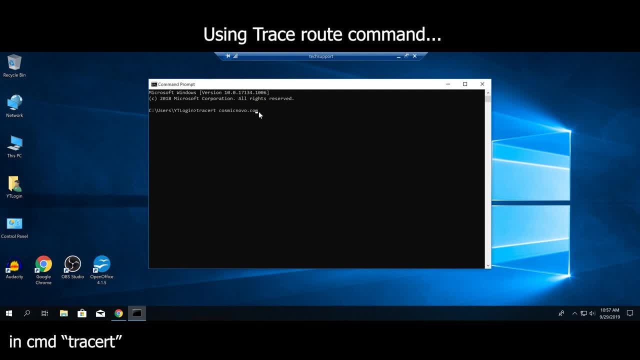 As soon as I hit enter here we're going to see what happens And I'm going to explain all the steps that it's going through. All right, Hitting enter, We trace out executed. This is typically what happens. It takes maximum of 30 hops. 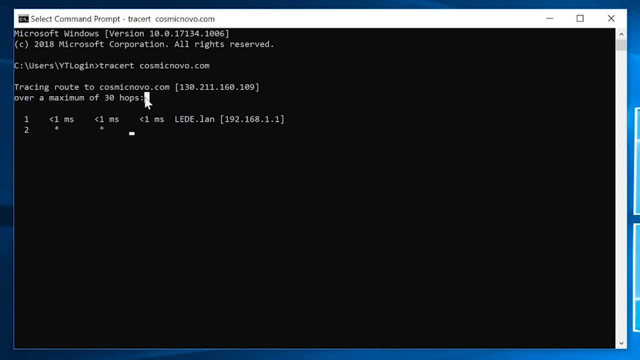 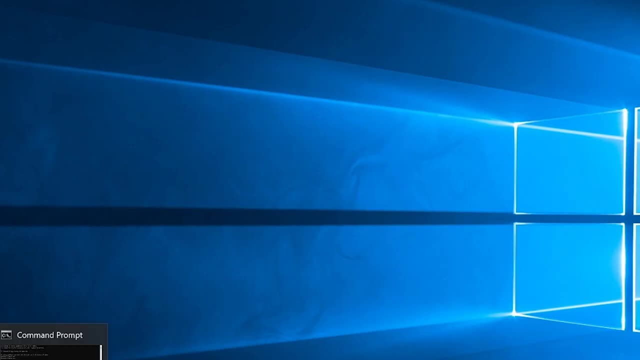 And 30 roads, or 30 paths, if you will, in order to reach the final destination, which is this IP address for this website, And this may take a while. This is why I have a finished TraceRT of all the routes taken for that website, And I will show you what that is right now. 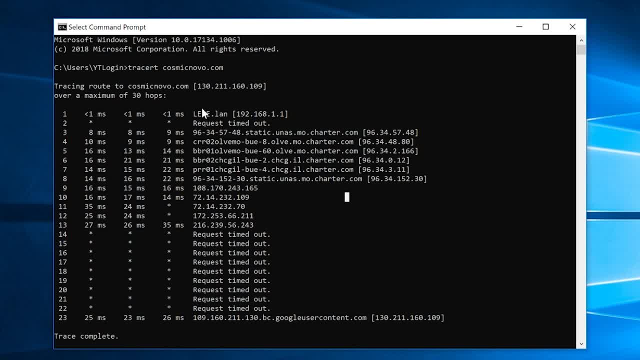 So let's have a look at some of the things that kind of stand out. The first thing, the first hop that shows up, is basically pinging my website. So I'm going to hit enter And I'm going to ping my IP address of the local computer. So the computer I'm using right now- local IP address. 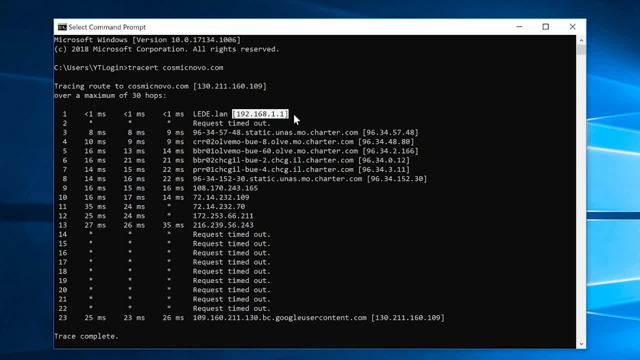 for that is 192.168.1.1.. So that's a typical local IP address. Second hop is basically trying to ping my IP address, external IP address for the internet. So my internet provider, which is Charter, is actually blocking that information for security reasons. It automatically blocks it. 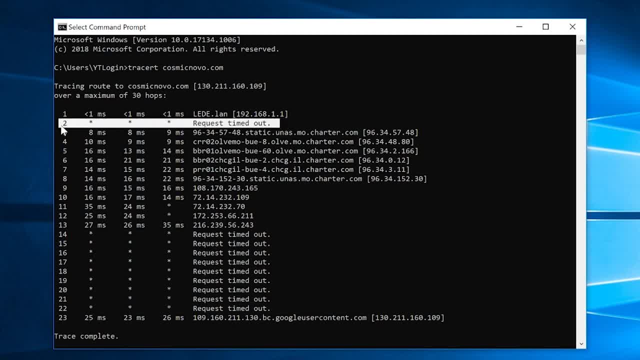 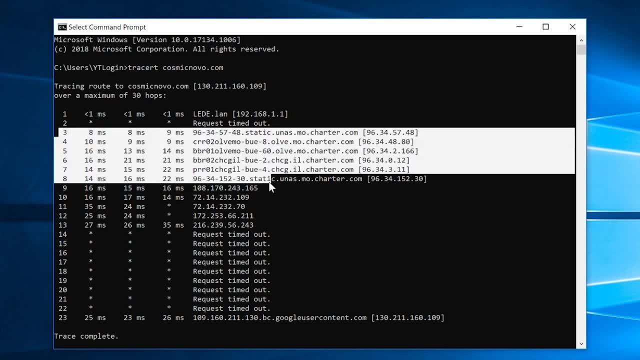 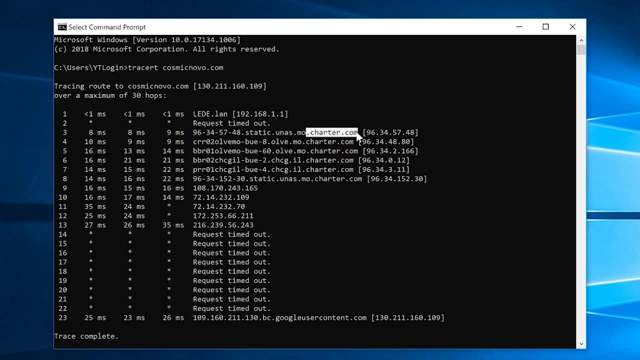 There's nothing I can do about it, But it's perfectly normal to see a second hop fail timeout like this, And then you can see that hops three through eight are all from my internet provider, Chartercom. Charter is my internet provider And you can see all these if you will switches. 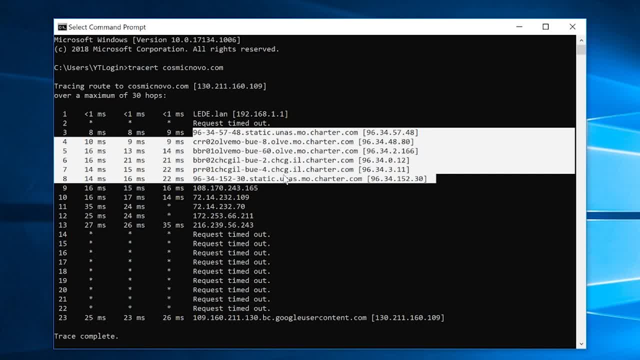 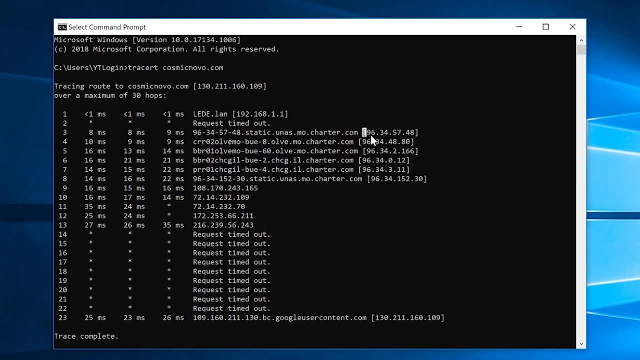 that it takes in order to access the internet. It goes the outside of the internet, So the Charter's network, So it goes through all of these And it seems, everything seems fine. So that's perfectly fine. And then finally reaches the internet, And then it has to go through this. 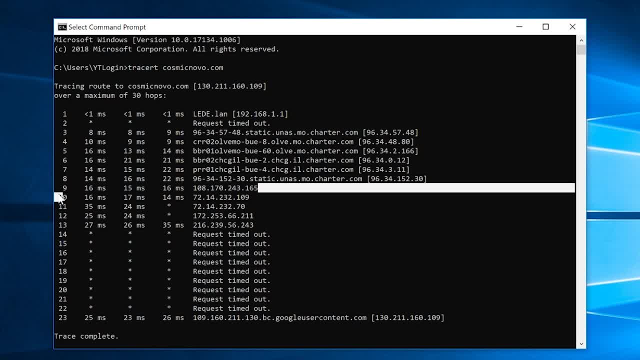 switch here And again it looks normal. This route is normal. And then it goes to the number 10.. Again it's normal. Then we look at 11. And we can see that there's increased millisecond response- Not necessarily too bad, because we're not talking like 80,. 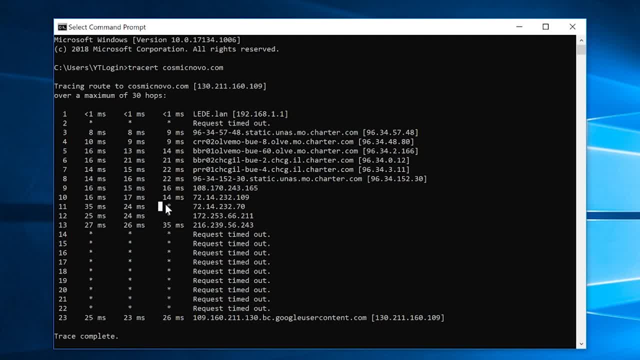 milliseconds, 100 plus or something like that. However, something does stand out here, and that there is a third. on the third response or third attempt, ping of it is: there is no response whatsoever. It timed out. So if we are having issues connecting to the final destination, 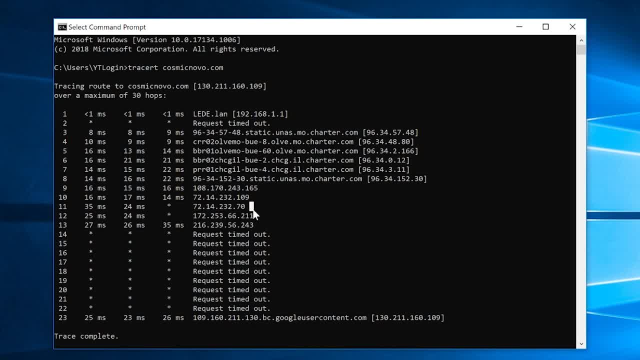 potentially we could look at the switches or servers that are located at these two IP addresses. So the first one is 7214.23.. 232,, I'm sorry, .70. And this other one that starts with 172.. So, because we see no response, 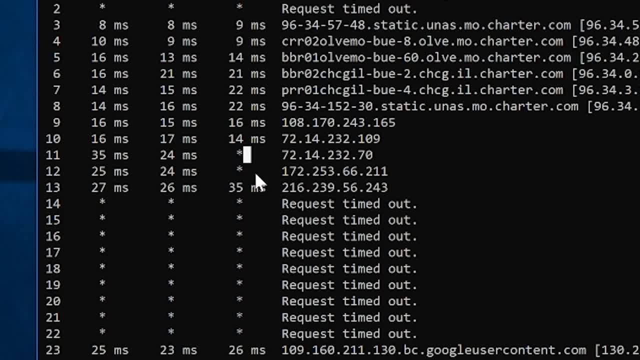 here at all for the third ping there. we can kind of possibly assume that there might be some kind of a latency issue with these two switches, or nodes, if you will, or they could be server or whatever it is that they are. We can look at that because it could be a server somewhere. 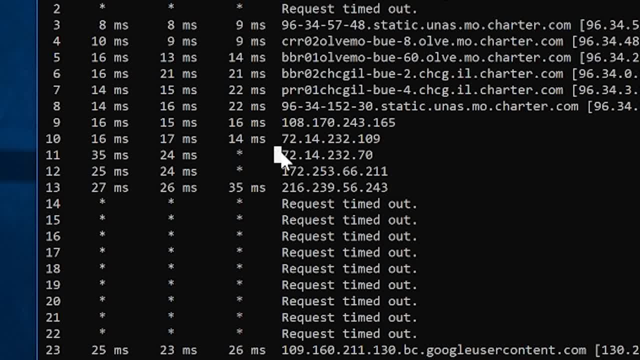 And the reason I say server is because it could be a server or whatever it is that they are. And the reason I say server is, in a sense, depending on which type of thing are we troubleshooting. Are we troubleshooting a website? Are we troubleshooting application connection? 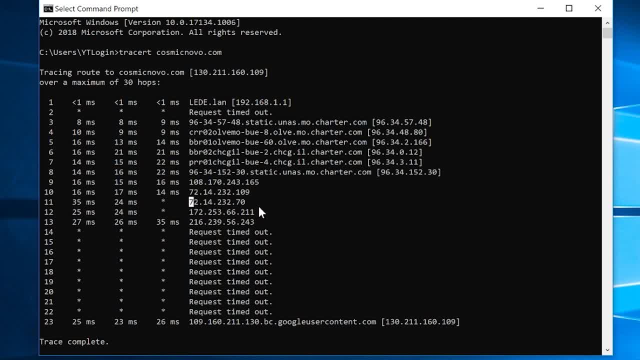 this and that, So it could be a you know part of the final destination of like, for example, application that maybe uses some kind of database that is located at this server or whatnot, Or server itself could be the firewall. We don't know, But we need to know, kind of what's causing this. 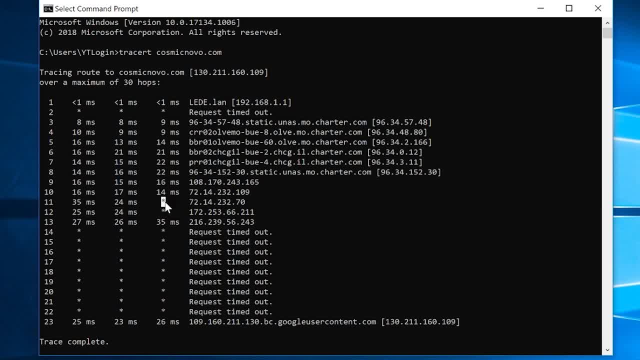 you know, delay Or lack of response whatsoever. if there is a problem, right, But typically that's associated with higher millisecond response time. So in our case this is probably just normal And chances are that these servers here just have a limit of how many times you can ping it. So we're going. 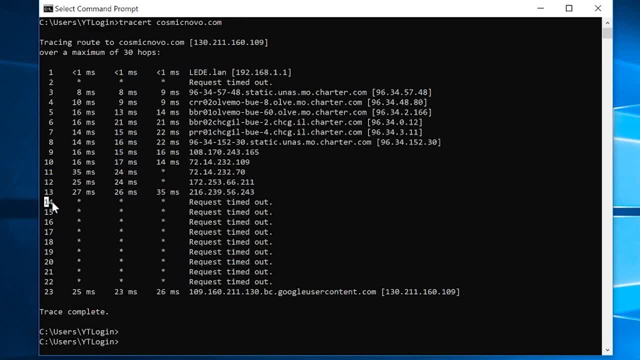 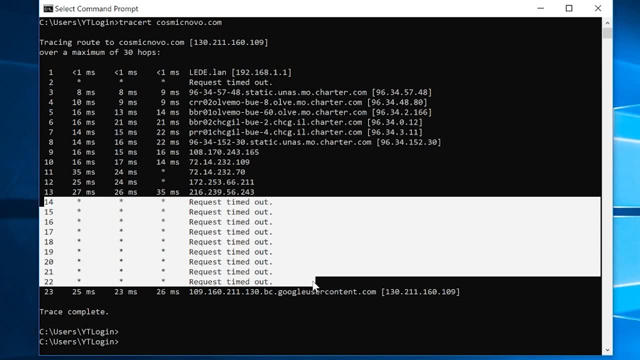 to move on from that. And then it goes through a bunch of different nodes here which could mean that it's just blocking. This is very typical, that these nodes are literally just blocking These type of connection requests, which is fine, We can. this is pretty normal. But every time you 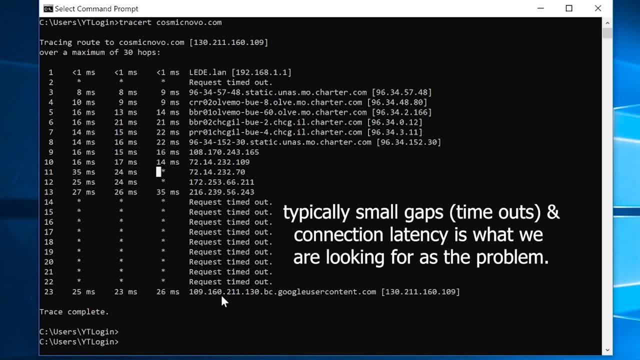 see a gap in between, where it fails somewhere. this is something we would have to be concerned about, And we'll potentially look at that here in a moment. But this is an example of a good trace route response. And then finally reaches the destination of 130.211.160.109,. 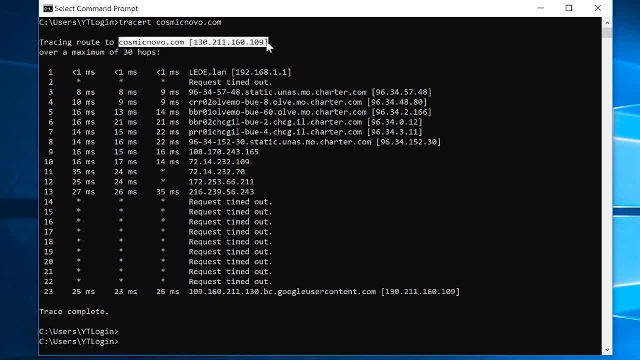 which is where CosmicNovocom is located, as you can see here. So it took all the routes and it took it 23 routes to get to the final destination, And we know that everything is okay here, All right. So I found a website that's supposed to be down, a safe website, And let's see, do I have? 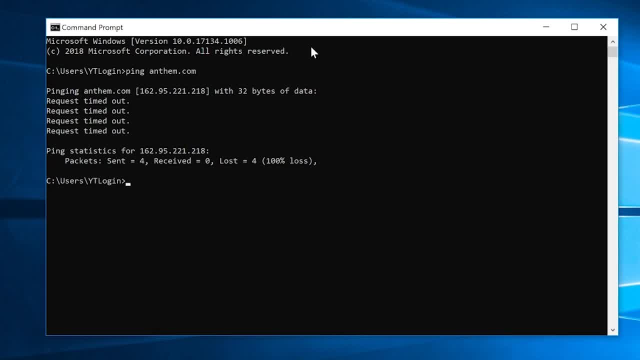 that going here. Yep, I had it tested. It's Anthemcom, which is basically insurance provider, health insurance provider, And I saw that it's down. Let me just double check here one more time. I'm going to ping it one more time to make sure. 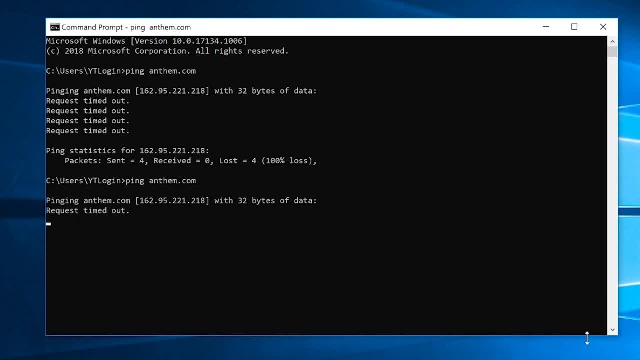 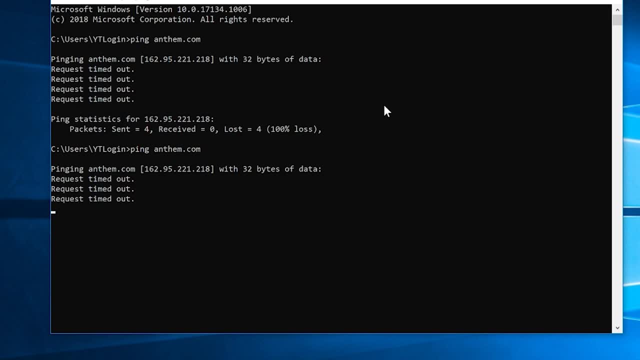 that it's down, And then we're going to do a trace route on it to see if we can figure out what's causing the problem. Chances are it's the web server itself, but it could be something in between too. So I'm going to do a trace route on that as well, And then I'm going to and you can. 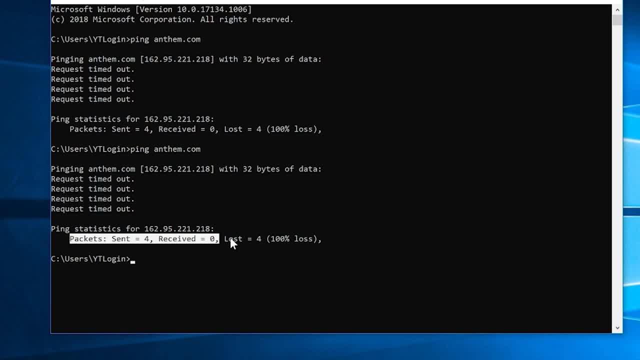 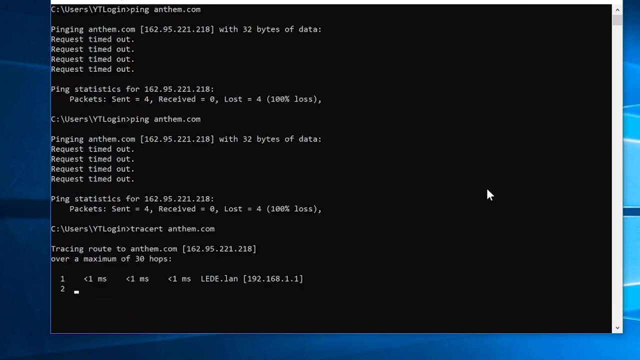 see that it failed. You know, sent four, received zero. It's time So we're going to do a trace route, RT Anthemcom and see what kind of response we can get. Again, this may take a while, which I will just fast forward to the results so we can see what's. 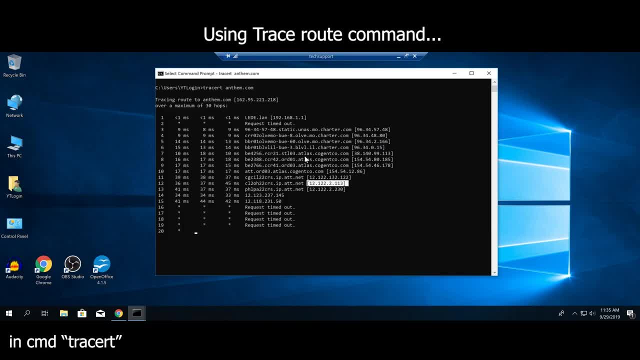 going on with that. So as we are looking at the results of Anthemcom, you can see that they are similar to what we had earlier. So we're going to do a trace route on that as well, And then I'm going to do a trace route on that as well, And then I'm going to do a trace route on that as well. 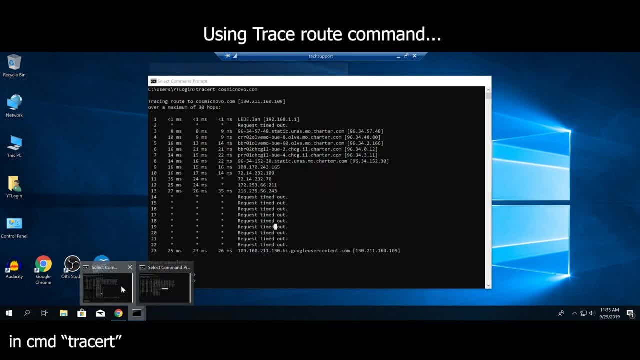 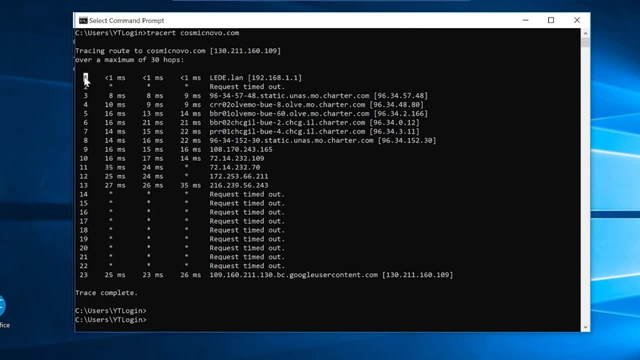 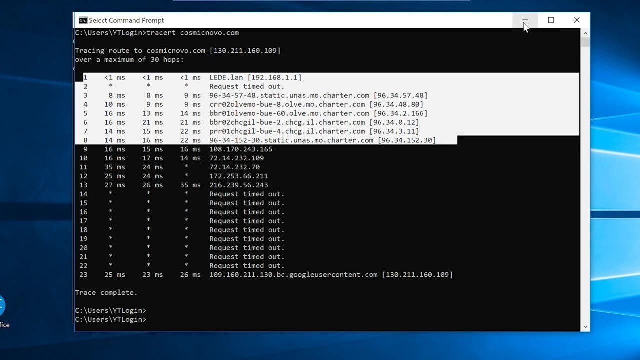 In the sense that it's taking same routes initially, And this kind of goes back to what I was talking about. See, this is the first one and we can tell that it takes, you know, hits my LAN, and then it goes through all of these charter switches. if you will And if we. 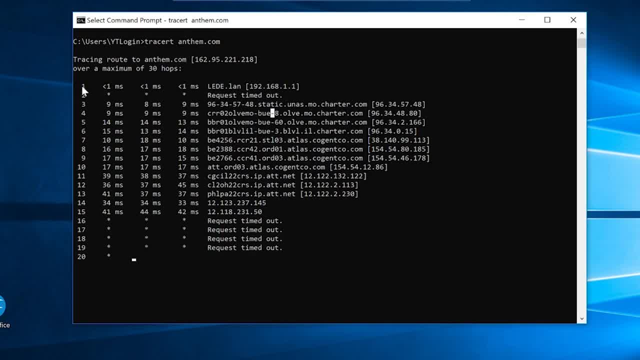 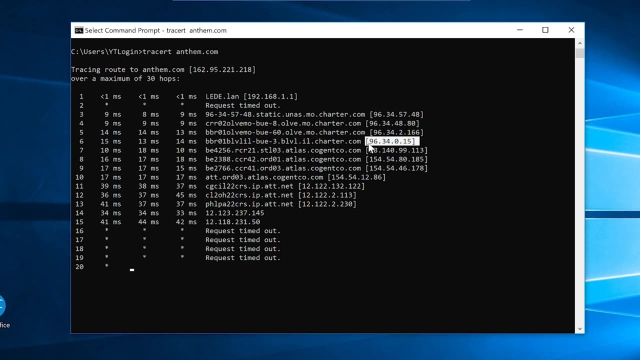 go back here, we can see that they are the same switches and it takes that same route. However, after it hits those, it decides to go another way, which was which was dictated by a. this switch, this, which says: okay, well, now we know, you're done with a. 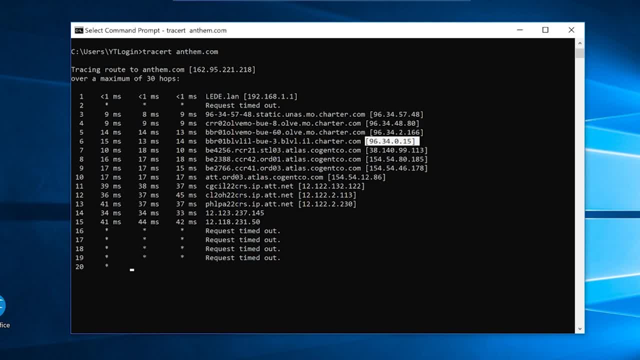 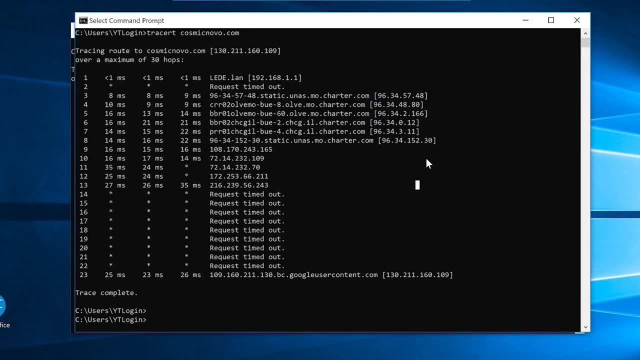 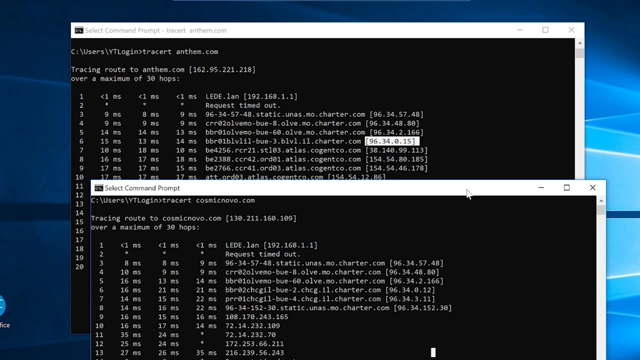 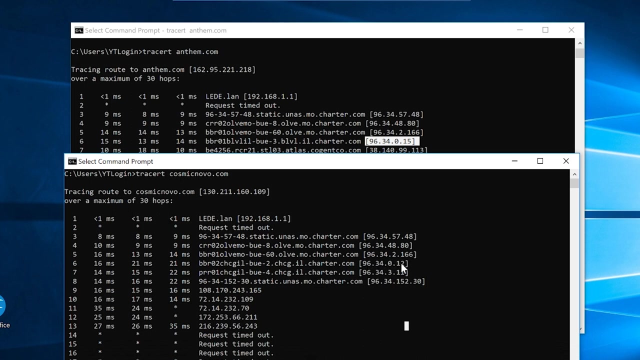 charter network. now you have to go through this, something else, so let's look at the previous one. i'm sorry, let's look at the previous one here. and did we take the same 15, 166? so, in our case, after the 166 charter, sent us to this other one which ends with 12 which, by the way, is probably 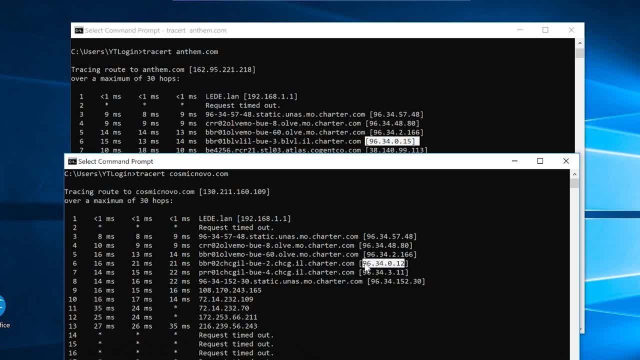 next to it. so there is a switch probably next to it in the same data center. you can see how it's only off by three ip addresses anyways. it decided in this case for the anthemcom, which is this top one, it decided to bypass the next switch, which typically would have been this one to route. 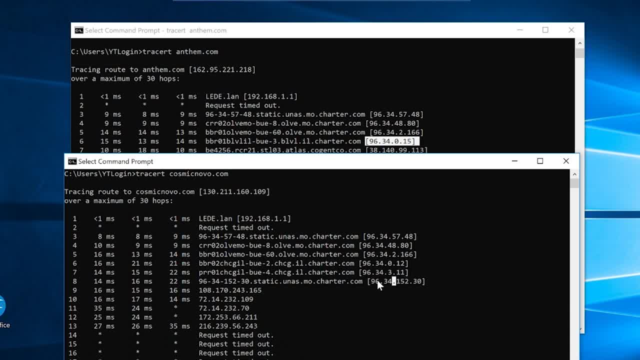 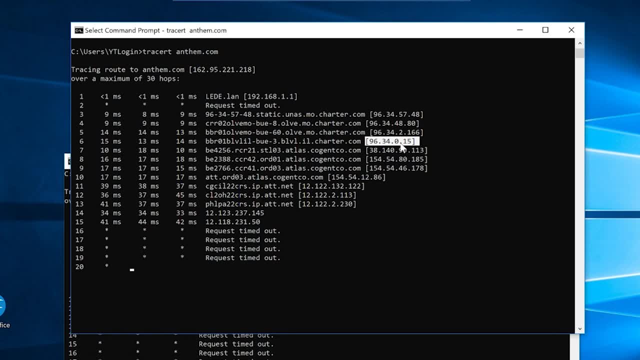 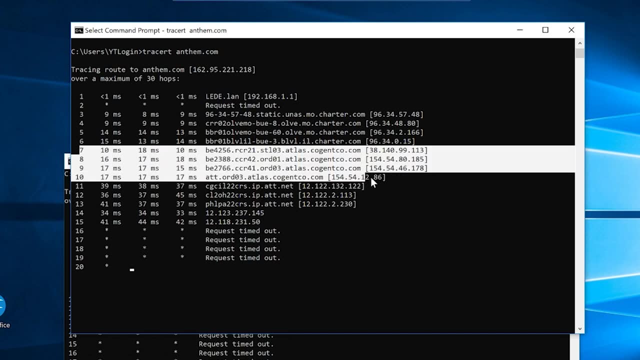 to cosmicnovacom. um, well, well, it had to take another one here, so instead of going to any of these other ones, you can see that this one just said: okay, well, this is going somewhere else and it takes a different route and it goes to this other, probably internet provider of some sort. 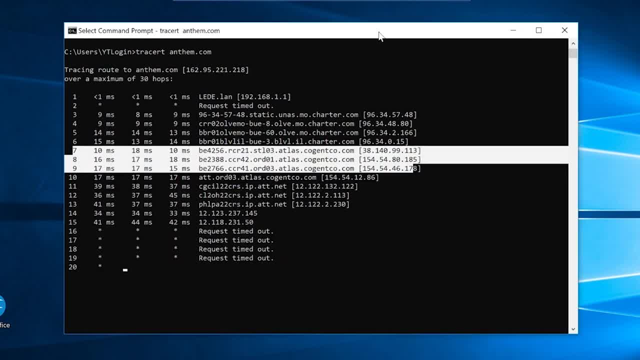 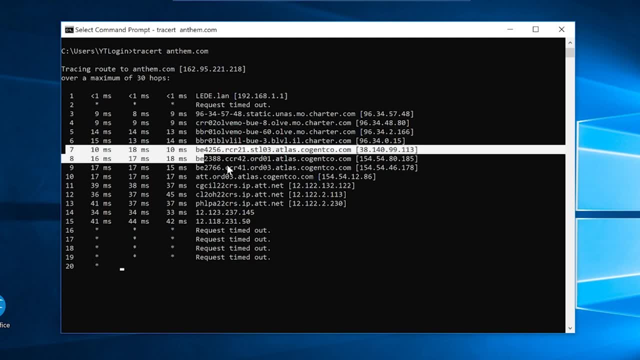 which i'm assuming is related to atnt and it doesn't say that here. but the reason i know is if you look at these seven through ten, you can see that the switches names are stl, which stands for st louis, ord probably stands for orlando, florida, and, uh, you can see that they're called atlascogento. 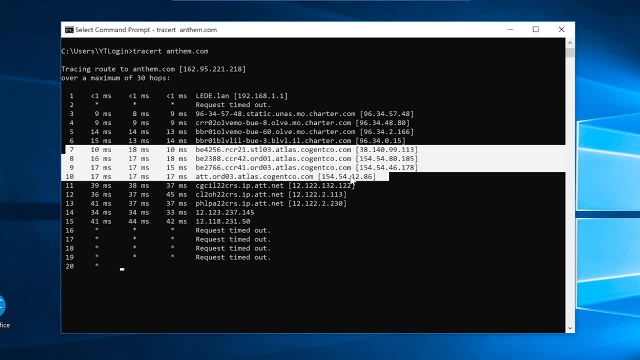 cogentcocom and you can see the ip address that are connected to there. however, if you look at number 10, you can see that it says att here, so which is atnt, probably orlando, so it goes through florida somewhere and then it continues with switches that are located or that are that belong to atnt, and then 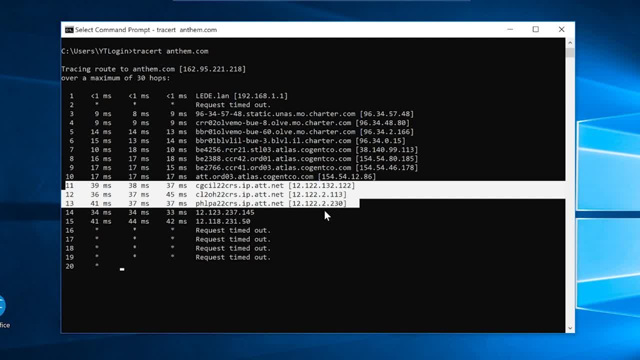 routes it further and you can see that it hits another three gateways, uh, most likely um in uh- on an atnt server, before it reaches its final destination. this is still taking forever, so once it's finished, i'll i'll show you, uh, what the end result is for anthemcom. however, i want to 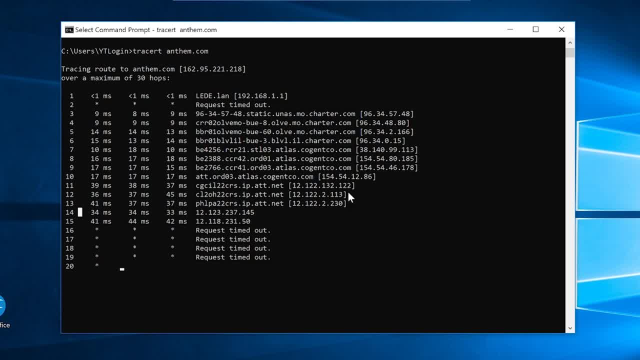 talk about a point of failure that may occur, that may show up in trace route command, and here's a really good example. we can look at these atnt switches here. so 11 through 13 trace route is can tell you immediately whether something failed and in the path that it's taking, so it's. 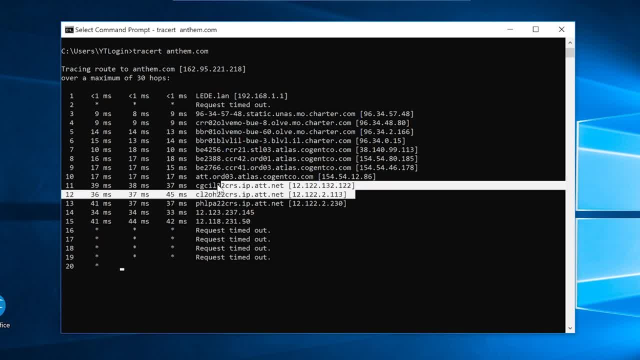 we can imagine that in this example, that actually it's done. so let's pretend that the data that's being sent out here is being taken literally and we can see that this data is being sent out here in the path that it's taking. so let's pretend that number 12 here timed out. so let's pretend this one timed out, literally timed. 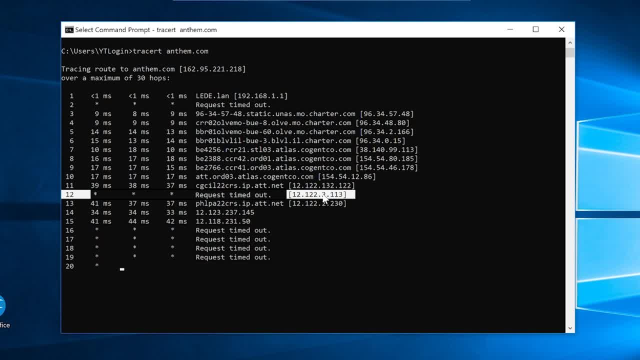 out and we need to figure out: where is it at who? what's wrong with this genstar if it timed out that either it's blocking the uh, this type of uh information from being sent back, which happens with kind of by intuition, that it's supposed to take another route because it goes to the third one. 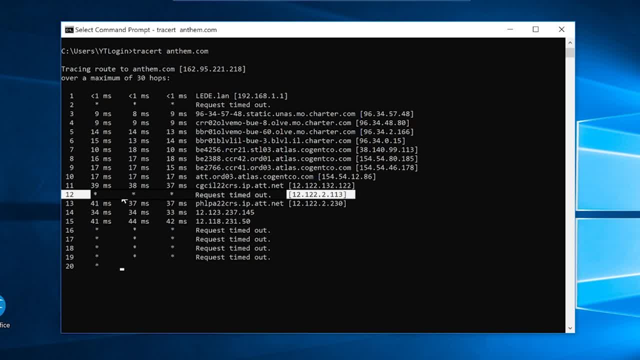 here, but for some reason, just one, this one in the middle, times out. that's a clear indicated of a switch that is, or the switch that is just bad. so how do we find out, you know, if it's bad or not? well, we would have to reach out to this guy or this company and ask them: okay, well, we need to. 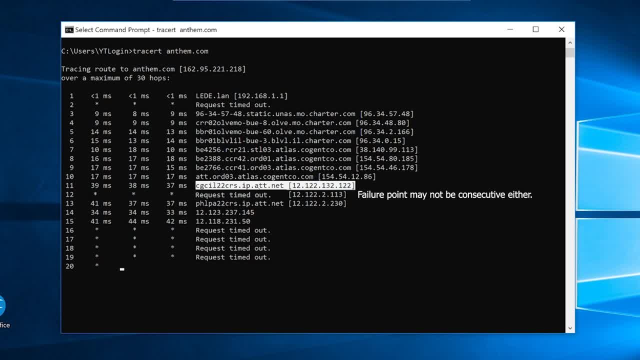 get somebody from AT&T on the call or call them or contact them and say, hey, there's a problem here. and they'll be like: okay, well, let's send me the results of traceroute from your location and they send it. you send it to them and then suddenly they're like: oh, the number 12 failed. 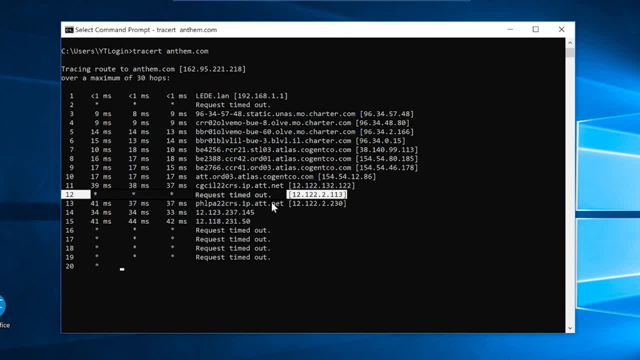 but we still know it's kind of on their network because it keeps going to their network. you see what i'm saying. it goes to AT&T. we know all three of these hops are going to go to AT&T, be at&t, but the middle one fails. that means it's still on their network and the problem is on their. 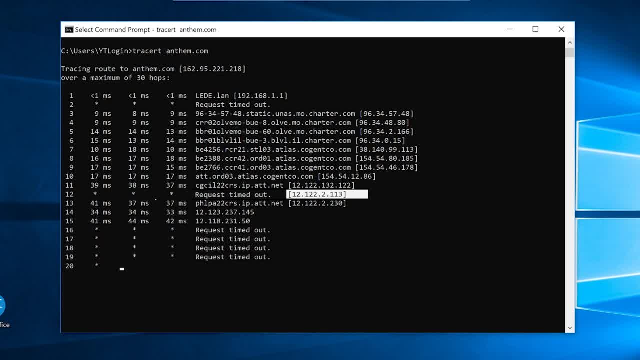 network and they need to look at this and they would know it would. i know it would say timed out here, but they would know what the next one would be or should be, or whether there is a break of some sort that prevents everybody and that one switch is causing the problem. so they would look. 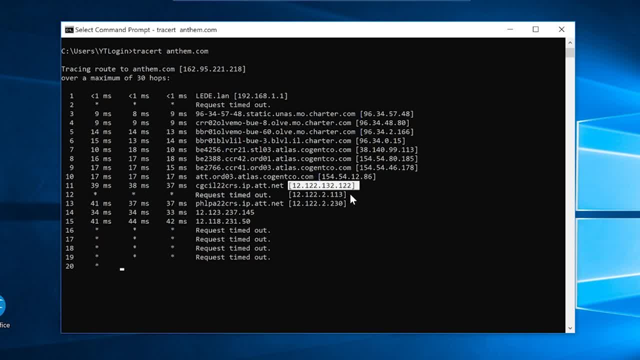 at this and they say, okay, well, we know it's on this network, let's scour our network and look for this broken switch. and that's the point of trace route. of course, there could be other examples of that, and that is, let's say, this one doesn't time out, but there is a huge, huge latency issue here. 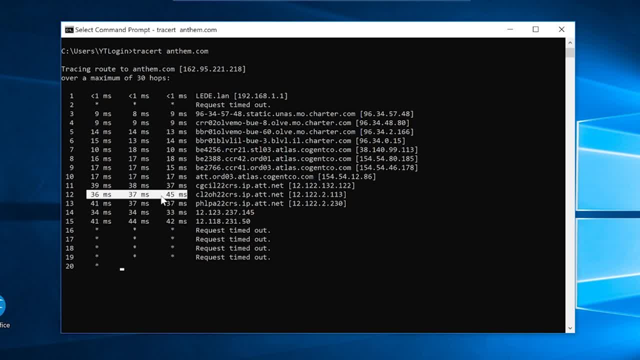 that would also indicate- that would also be indicated by trace route- that there is a problem. so let's say the response time is like 100 milliseconds or even 80 milliseconds. this caused connection timeouts on the application and or a user end as well. so let's say there's a huge latency here. there's another reason why they would. 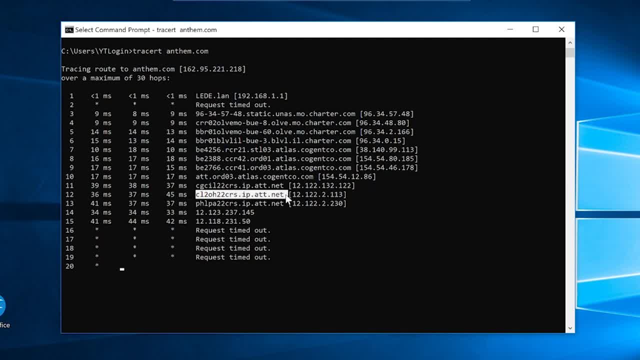 want to look at that switch or server and kind of see what's going on. the reason i say server because it could be the final destination. we don't know, but in our case we know it's not. it's just a switch that it's taking and then with the trace route information we can send. 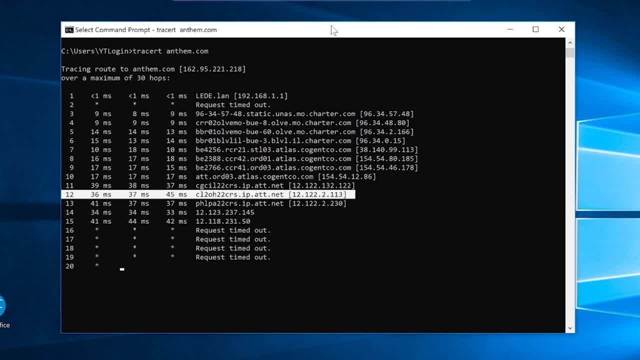 forward this information to them and say, okay, well, you know. this is probably what's going on. now this thing is going to time out and i'm going to kind of tell it to skip by hitting enter the attempt. for some reason, it gets stuck like this, waiting to get a response from the switch. 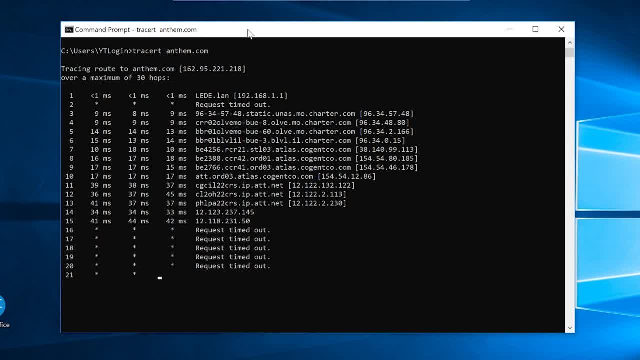 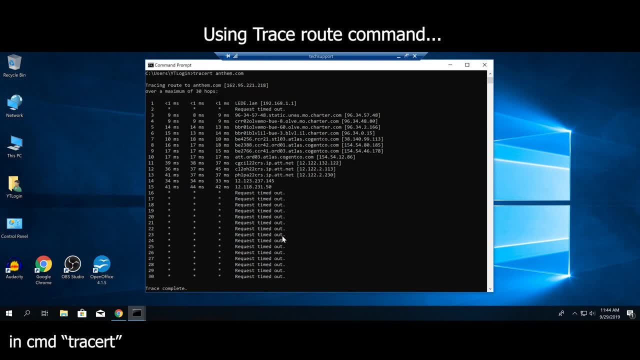 and then i'm going to fast forward this to the end result, so, as the final result of the trace route is coming up, we can see that the anthemcom is just simply down. this is what it tells us, the normal response from the trace route when everything's okay. 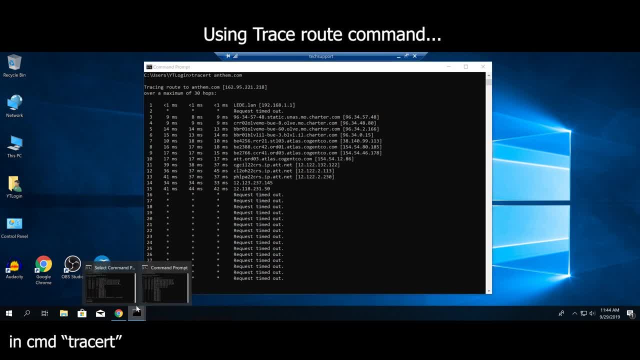 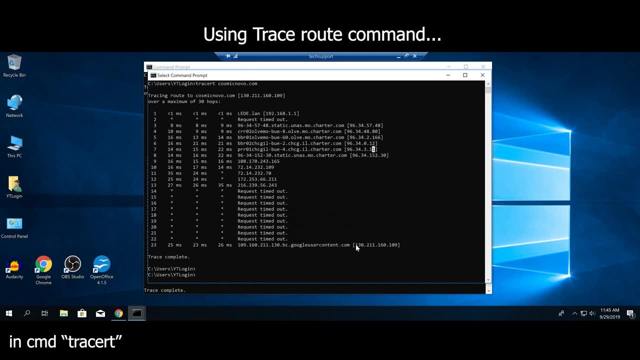 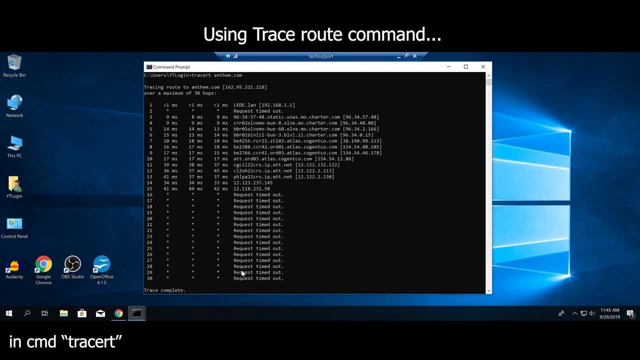 is indicated in my other window here and you can see that the final hop gives us the final destination address. in our case of anthemcom, it doesn't, it never reaches it, and this is clear indication that there's something wrong at the web server level. so the webmaster for anthemcom 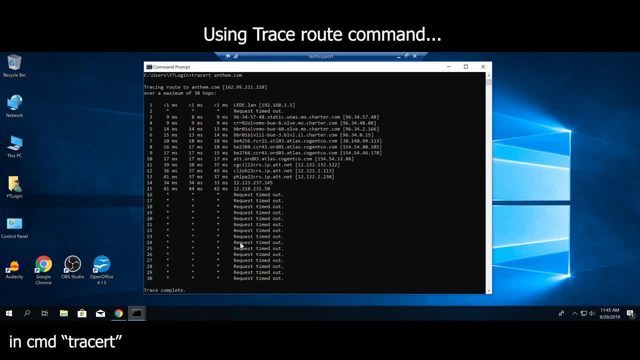 needs to look at it and resolve the issue at the server level. so but you know, when we know that the website is down for everybody, this is not necessarily the reason we would use traceroutecom, our traceroute command 4. we would simply just use ping command to see if it's up or down. but if there 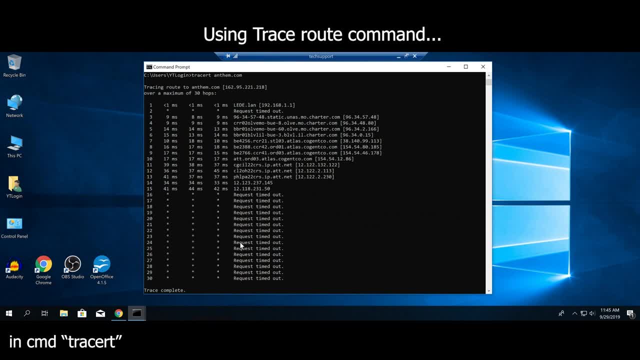 is an issue of latency. if there is an issue of website or an application working for some people but not others that are on a different network, that's when we would use the trace route. so it's for troubleshooting connection issues that are specific to a network. you know meaning that. 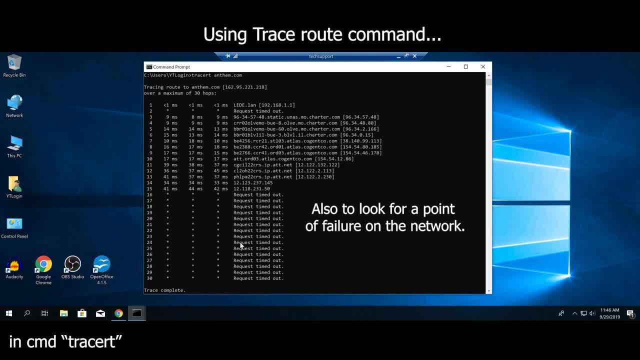 just because i can reach it doesn't mean that some other people can as well. so this is how you would use trace out to figure out where is the breaking point on their end and why can't they reach, or why can't i reach a certain web server. 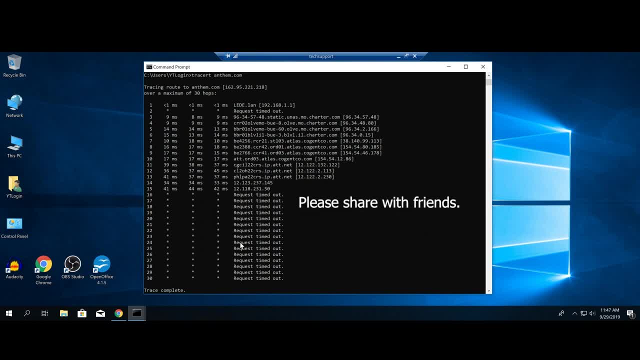 application server or what not? please share this video with friends, leave a like or any comment and i will answer them. thank you so much for watching. have a good day, bye.